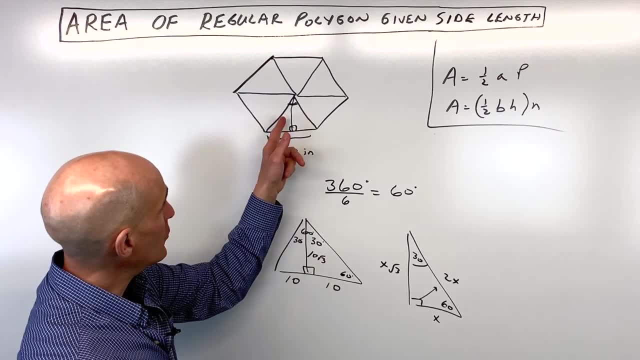 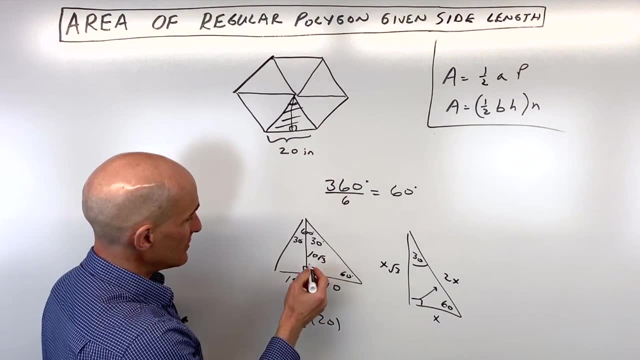 x squared of three. So if we want to find the area of this triangle, which is this bottom triangle, right here, we just have to do: area equals one half the base. okay, so the base is 20, times the height, which is 10 squared of three. And then all we have to do